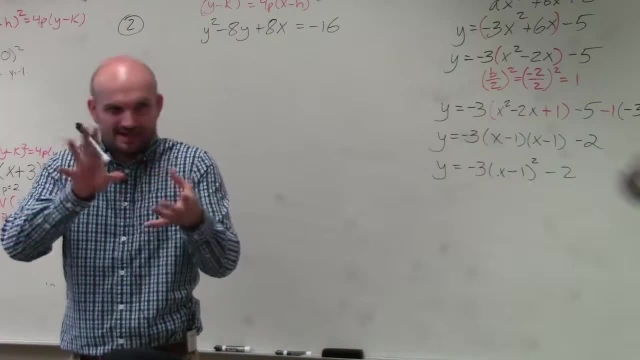 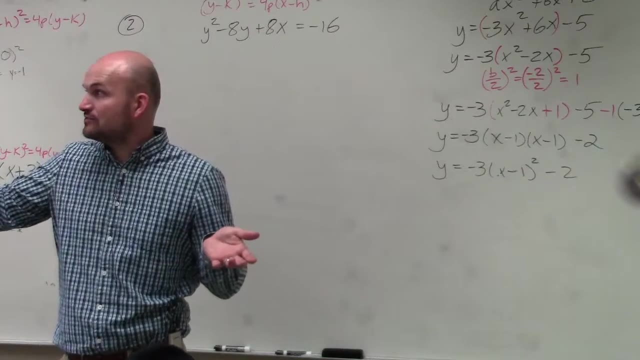 was. those were in kind of conic's forms. We just kind of had to arrange them a little bit, but they were in conic section form, whereas these equations don't really look anything like conic section's form. What we're going to have to do is now complete the square. 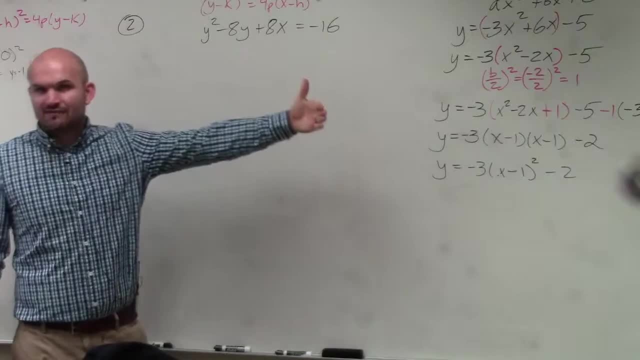 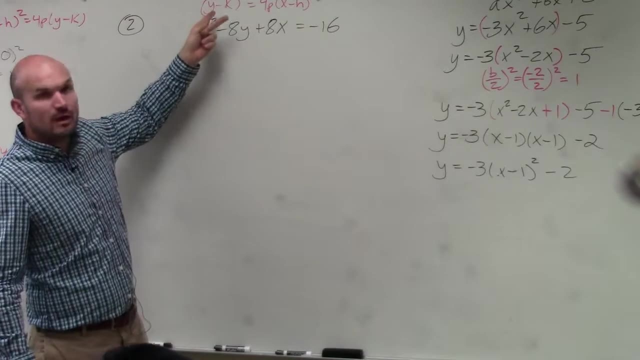 to get into that format. So again, just like I did in the last time I taught, I said: guys, write the equation that it's supposed to look like Y is squared. so I wrote the Y squared equation. right, If X was squared I would have wrote the X squared equation Really. 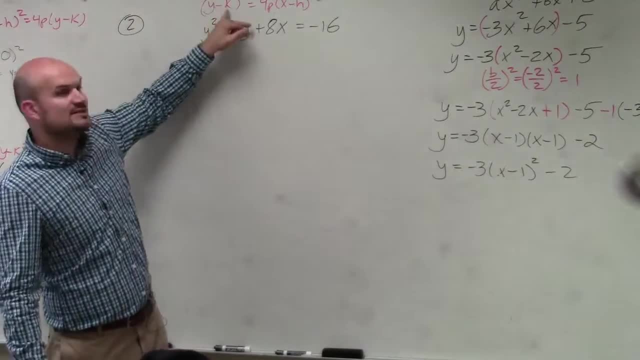 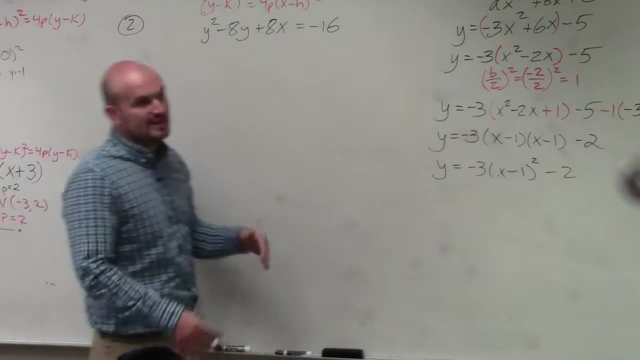 the big difference between the X and the Y squared is: remember Y is always with K and X is always with H. So you just got to remember that, All right. Now notice, do you guys see how the Y's are on one side? the X's are on the other side, Right, 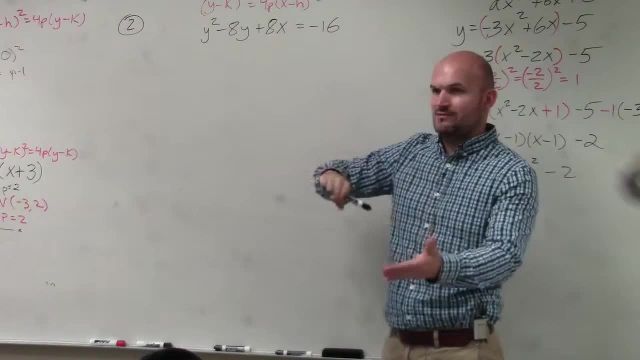 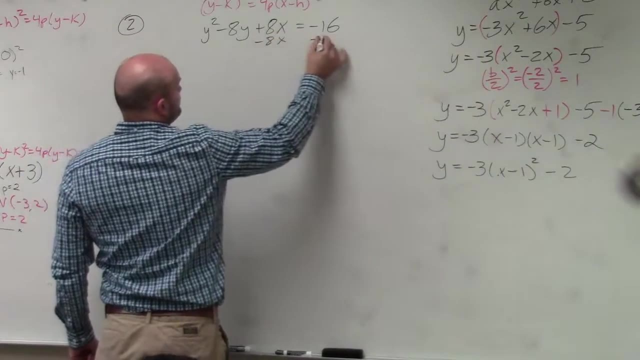 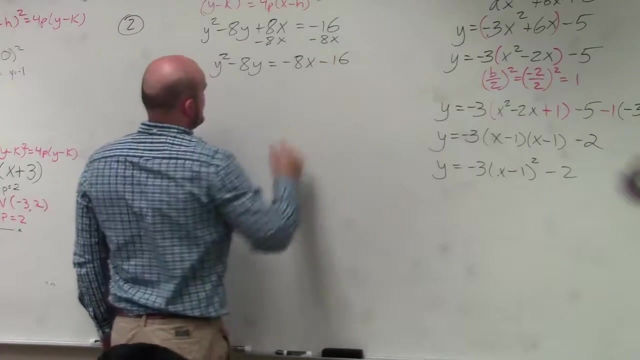 So what I'm going to do then is get the Y's on one side and the X's and whatever that four P number is on the other side. So I'll subtract an 8 X, So I have Y squared minus 8. Y equals negative 8 X minus 16.. Does everybody see that? 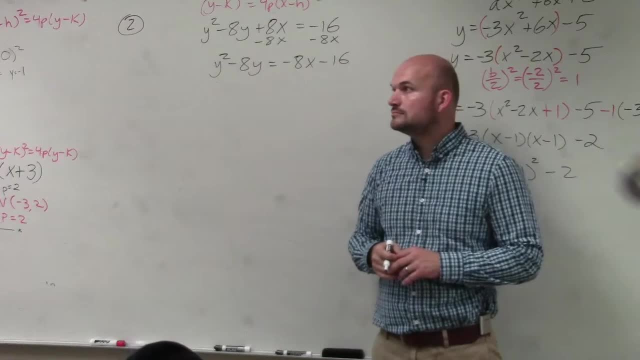 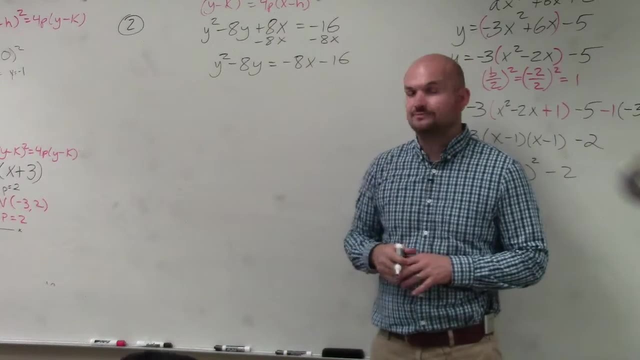 Do you know white squared? Huh, You're doing Yes, All right. So now Need a new formula. All right, We're going to take our analysis arrangement, All right? So here's our formula. So let's look at how long does the trivial Shift зем? 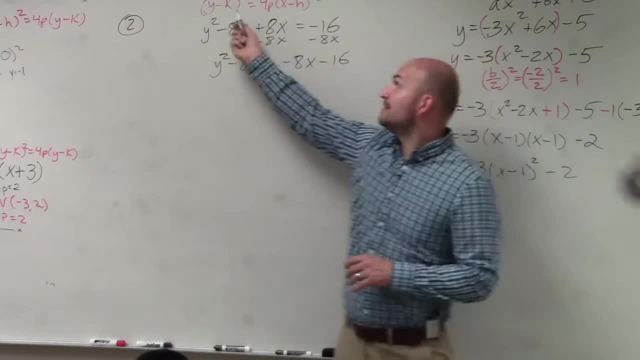 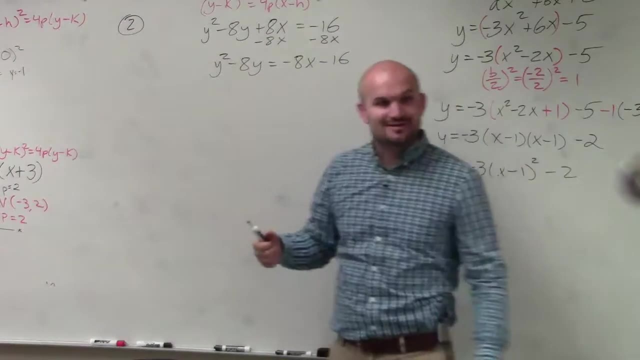 This is not a binomial squared. That is a binomial squared. I need to make that a binomial squared right. So to do that, we use completing the square. If you guys think about this, that's ax squared plus bx. 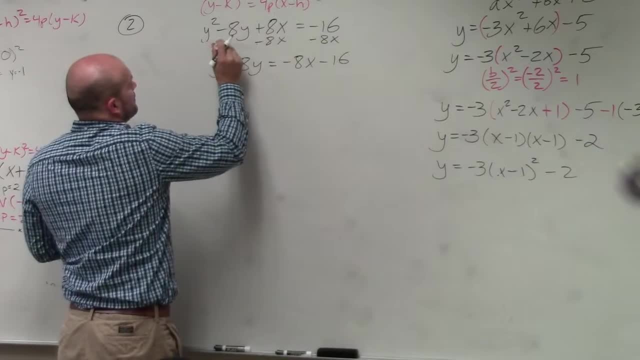 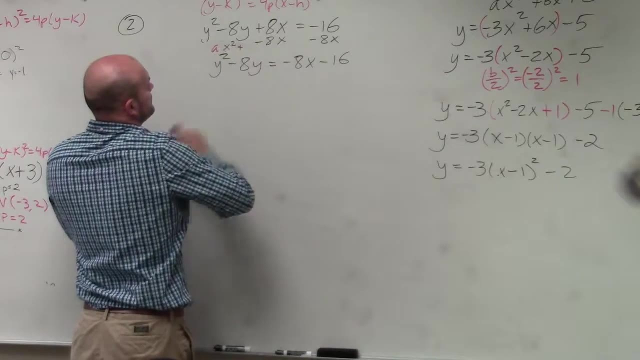 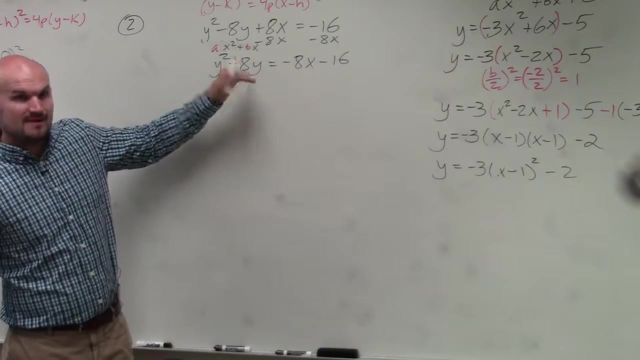 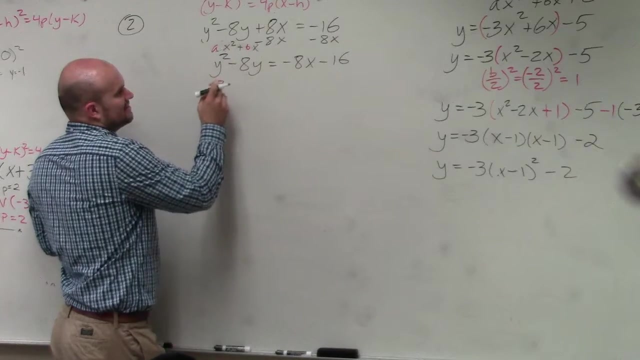 Actually, let's do this in red. Do you guys see how that's a quadratic? and I have a and b right? So if I have my b, I can find the value c That completes the square. So I just take a negative 8, divide it by 2, and square it. 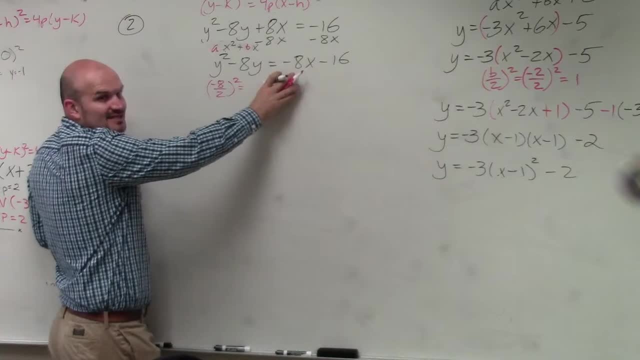 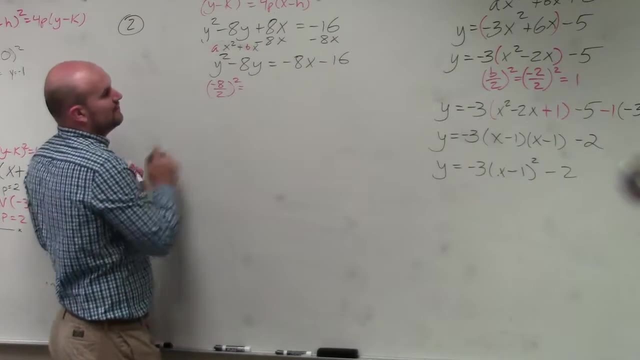 Now I can't complete the square on the right side because x is like linear, not quadratic. Does that make sense? So I can only complete the square here. So negative 8 divided by 2 is negative 4.. Negative 4 squared is 16.. 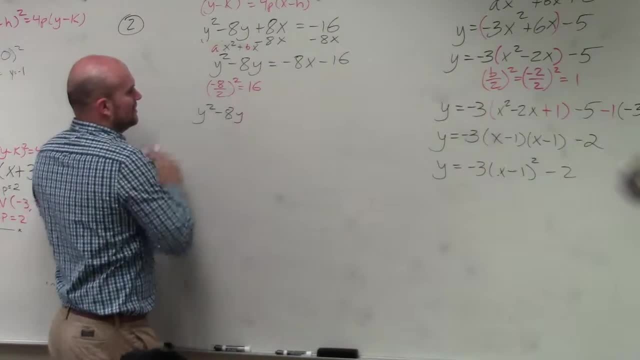 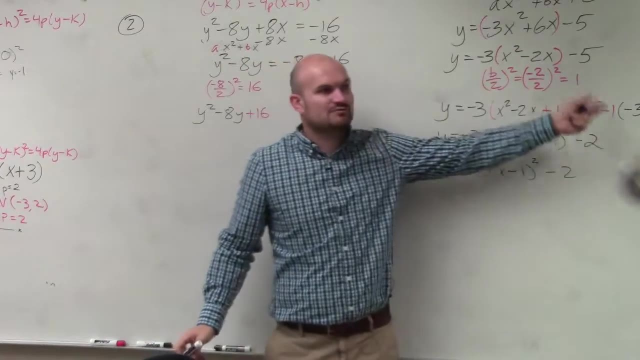 Now this is where sometimes students get confused. Remember when we were completing the square for these, for quadratics, I added and subtracted on the same side, right. Well, in this case I don't want anything on the left side. 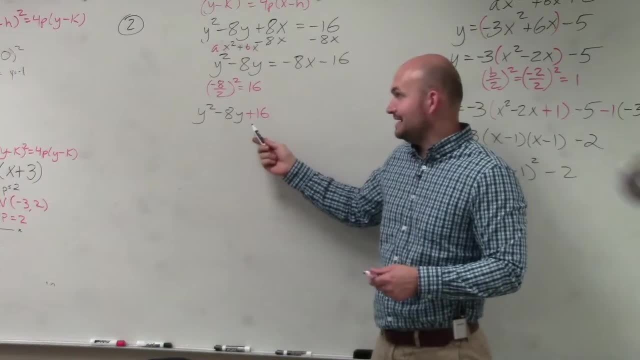 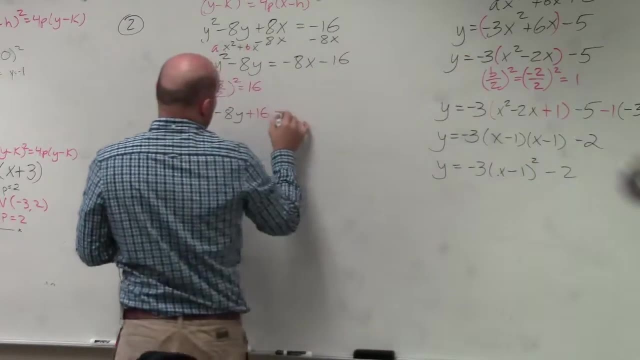 except for that binomial squared. So if I add 16, inside of here, I don't want to subtract 16 on the side, I want to put the 16 on the other side. So what I'm going to do is I'm going to add a 16 on the left side. 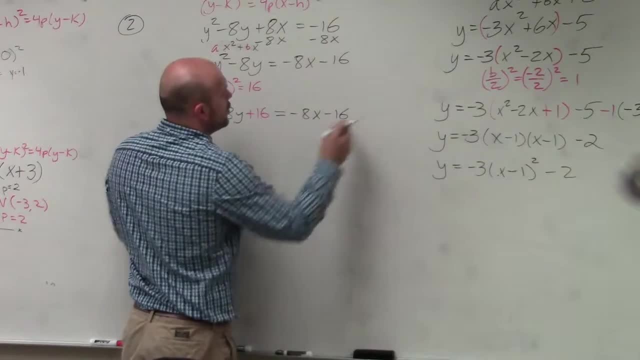 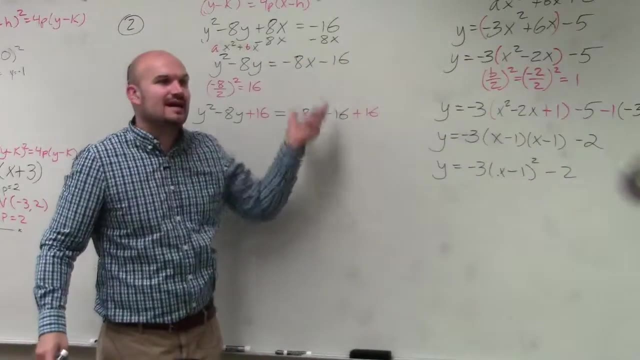 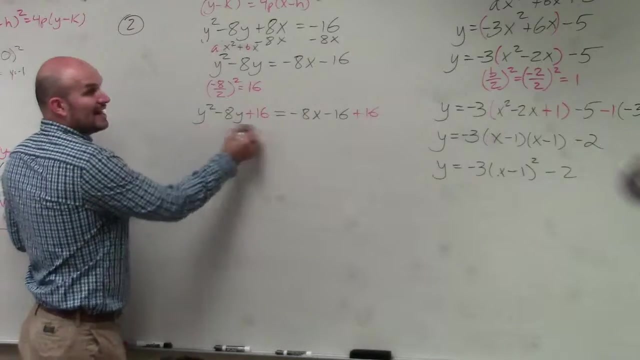 and I'm going to add a 16 on the right side, because adding and subtracting on the same side is equivalent to adding on both sides. right, I still kept the equation the same. It's still balanced. Then I created a perfect square trinomial. 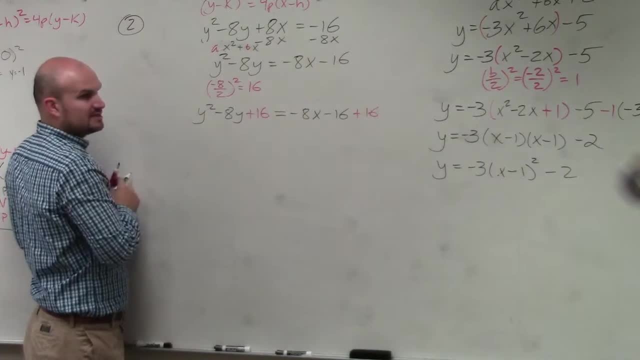 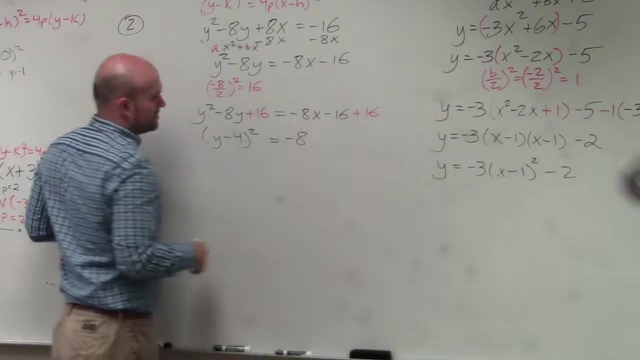 which can be factored to a binomial squared. what two numbers multiply to give you 16 and add to give you negative 8? And that goes to 0, right, So in re, Oops, that's x. Now I can't factor anything else out on here. 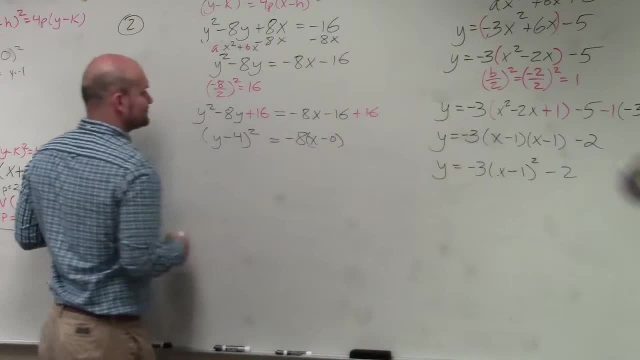 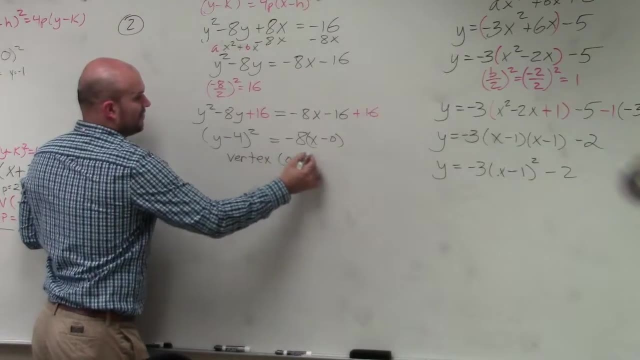 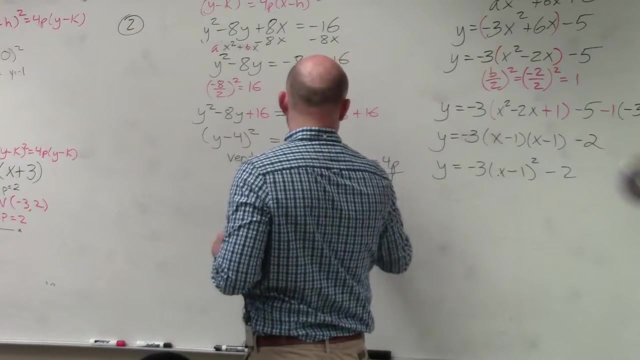 so you could say that's minus 0 if you wanted to. So therefore my vertex is 0, 4.. p negative 8, is equal to 4.. 4p. divide by 4,. divide by 4.. 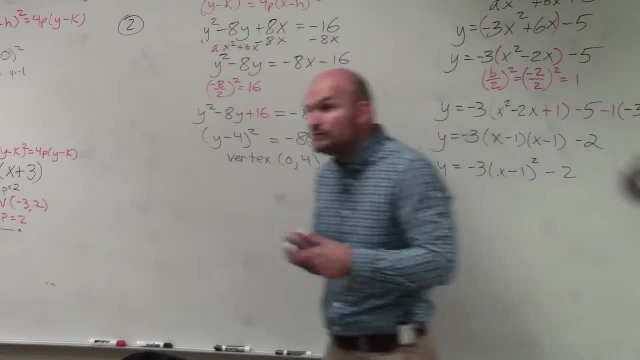 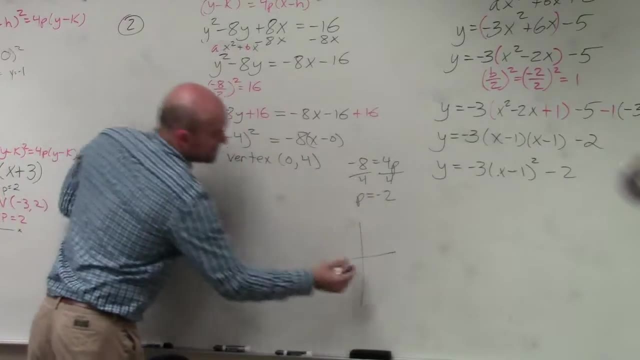 p equals negative 2.. Now again, people get confused. So again, sketch a graph. When you guys are taking your quiz, you'll have a huge piece of paper. Sketch a graph. I've got to rush in here. Vertex is 0, 4.. 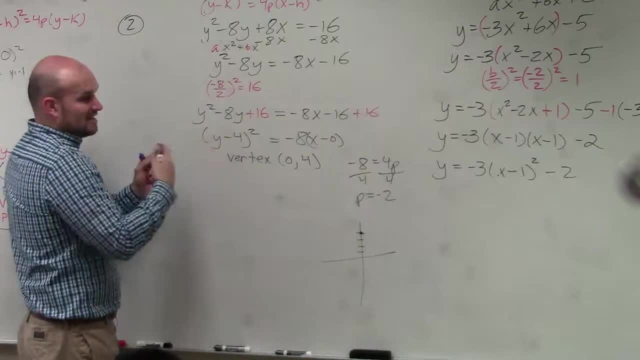 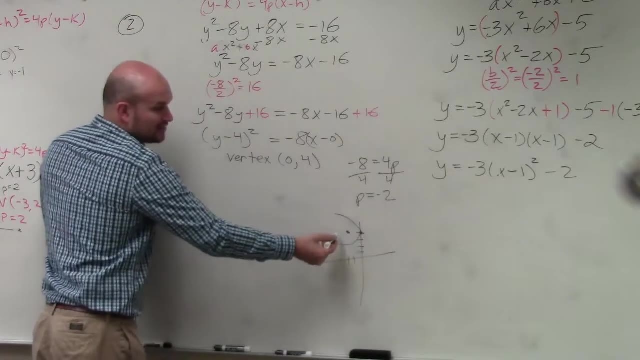 1,, 2,, 3, 4.. The graph y squared, so it opens left to right. p is negative, so it's going to open up to the left. So if here's 0,, 4,, if I go to the left, 2,. 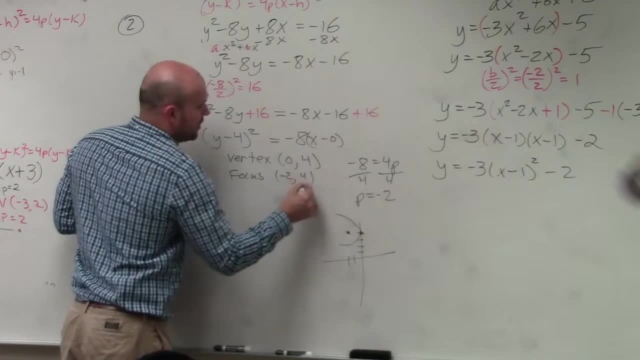 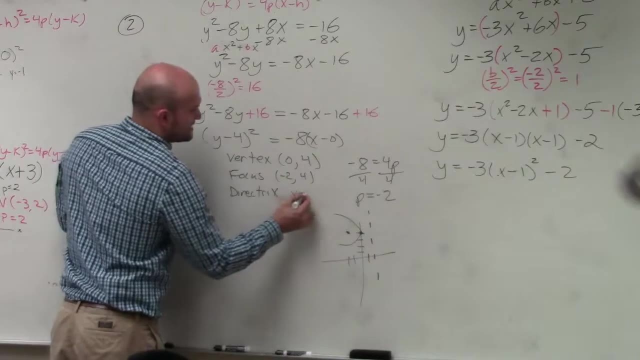 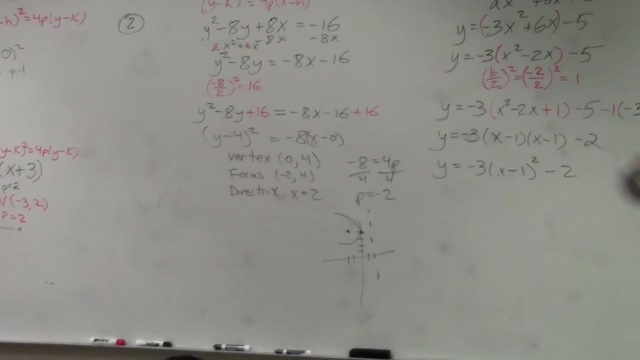 that means my focus is at negative 2,, 4, and my direction, Vectrex, is a vertical line over 2,, which is x equals 2.. Okay, Let's get that done. You guys have.